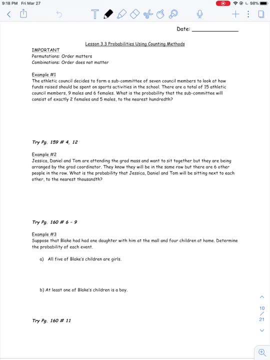 or a, C for combination, where order does not matter. So when we read the question, we're going to figure out if it's a permutation or combination first, before we continue. Example number one: the athletic council decides to form a subcommittee of seven council members. 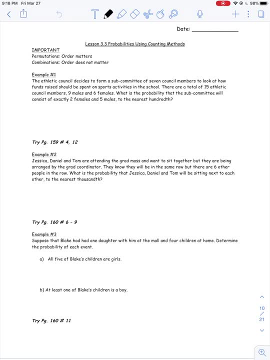 to look at how funds raised should be spent on sports activities in the school. There are a total of 15 athletic council members. There is nine males and six females. What is the problem? The probability that the subcommittee will consist of exactly two females and five males. 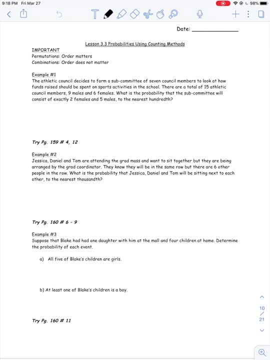 to the nearest hundredth. So in this case, when you're creating a committee, they're not telling you what jobs they're doing in the committee. They just tell you that they want a certain number of males, a certain number of females. So that would be a combination. 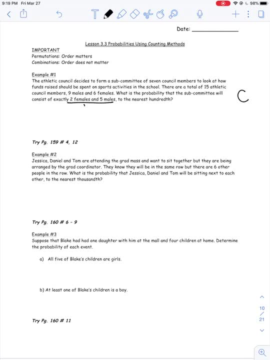 question. So we're going to use the letter C. So our want is the statement that they say in the last sentence. This is our want. We're going to identify members to sort out our type of homework or our type of order in the. 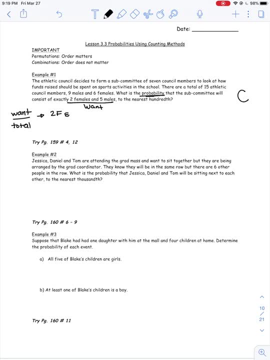 school. So whenever we're trying to answer this question of probability, we always have to write what, over total, our want is going to come from doing a committee of two females and five meals. So we would say: well, if I want to pick two females, I need I say how. 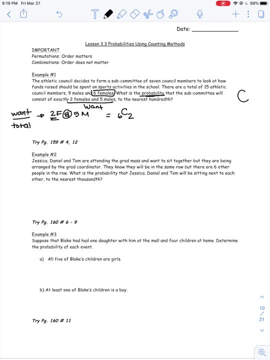 many are there. Well, that's going to give me. there's six females to choose from. From this information, two females, so it's going to be six. choose two whenever you see the word, and you are going to multiply. and now, from nine males right here, you are going to choose five males. so that's our want. 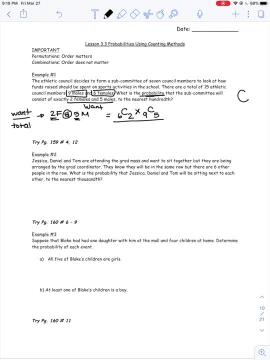 so that's what the actual statement wanted. now the total comes from saying how many people are selected, or how many people am i selecting and how many people do i need for the committee. well, the total. well, if i didn't care if they were male or female, there would be 15 people to choose from. 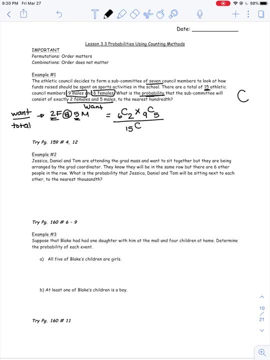 and i want to make a committee of. it says that you want to make a subcommittee of seven council members, so you're going to go 15, choose seven. so this is going to be our want over our total. so what we're going to do is we're going to put the top, the six, choose two times nine, choose. 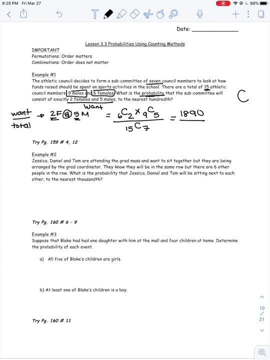 five into our calculator, we should get 1890 over. if you put 1527 you should get 6435.. now we're going to rate to the nearest hundred. so in your calculator you're going to divide these two numbers and you should get to the nearest hundredth would be 0.29. 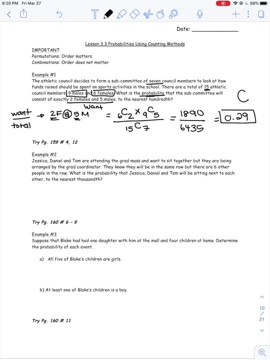 so that's our answer. example number two: jessica, daniel and tom are attending the grad mass and want to sit together, but they are being arranged by the grad coordinator. they know they will be in the same row, but there are six other people in the row. what is the? 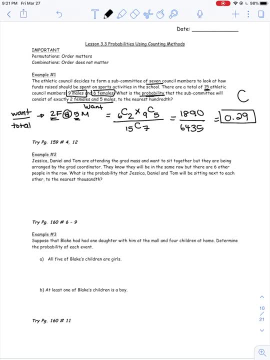 probability that jessica, daniel and tom will be sitting next to each other to the nearest thousand. so that means you're gonna have to have three decimal places. that's what thousand means. decimal places will be three, okay, so in this case we're gonna have spots to represent this, so we're 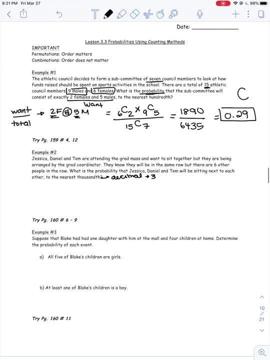 going to show what that means. we're going to have spots to represent this, so we're going to show what this looks like as spots. so we know that they'll be in the same row, but there are six other people, so there's jessica, daniel, tom and six others. one, two, three, four, five, six. so when i'm trying to do 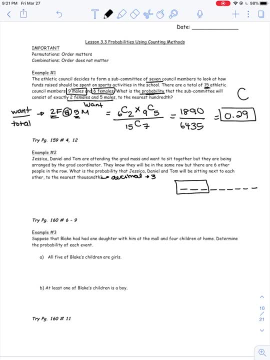 uh, trying these situations where people have to sit together, i'm going to put them in the first three spots just for now, and we're going to rearrange them by saying that there's three options for the first spot, because it could be jessica, daniel or tom. then if i put one person in, 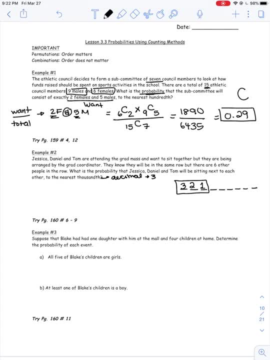 the first spot there's two people left, and if i place the second person, another person. in the spot two, there's only one person left. so that's going to represent three factorial. now the other people i'm going to rearrange by saying there's six people left, then five, then four, then three. 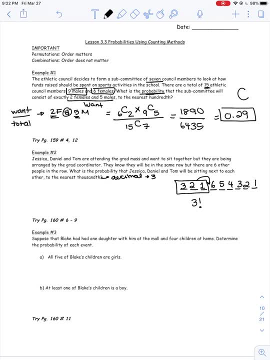 then two, then one. now, whenever we have situations where people have to be together, we need to say where they can go. well, they could be in the first spot in front of the six. they could be in between sixth and the fifth person, in between the fifth and the fourth, in between the fourth and third. 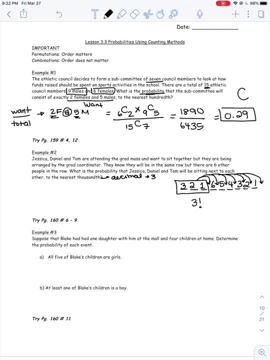 in between the third and the second, in between two and one and finally in the last spot. if you count all these arrows, there should be seven spots that they can go into. so you're first going to write six factorial, which came from all this, and then you're going to multiply. 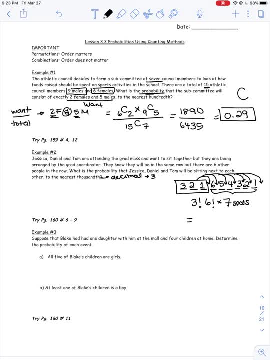 by the seven spots that those people could be sitting together in that row. so the another way of writing this would be three factorial multiplied by seven factorial. now, what we just did was we calculated the want. because of the word probability, we have to write want over total. so that's what's different about this lesson: our want is going to be. 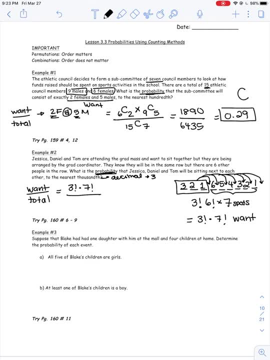 that 3 factorial times 7 factorial over the total is going to be. well, what if we just have to? what if there's no rules and we just have to rearrange these people in that row of nine people? because there's nine people in the row, so imagine you have nine spots. well, if 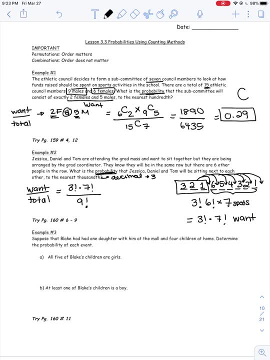 there's no rules. you can have nine people in the first spot, then eight, then seven, then six, so that's the same as saying nine factorial. okay, so we would put this into our calculator. the top would equal thirty thousand two hundred and forty, the bottom would equal three hundred and sixty two. 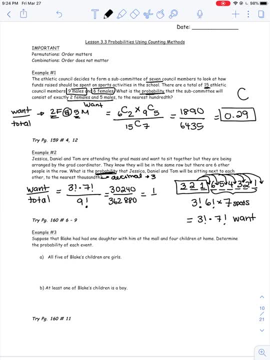 thousand eight hundred eighty, which simplifies: if you go into your calculator and press math, enter, enter, you should get the answer of one over two. so again, you're putting this into your calculator and then you're going to press math and then enter and enter again and you'll get that. it gives you this one half. 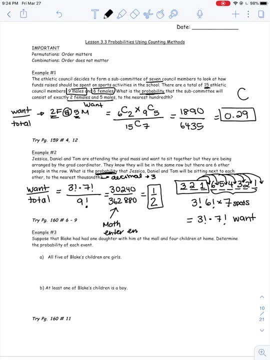 now we do want to write this. oh sorry, my bad, should not be one half. i was just checking my calculator, i'm just gonna erase this, okay, so 30 240 divided by 362880 gives me a. so it should be math enter, enter. it should have been 1 over 12.. i'm just missing 1 over 12.. which they want to say is one over 12.. 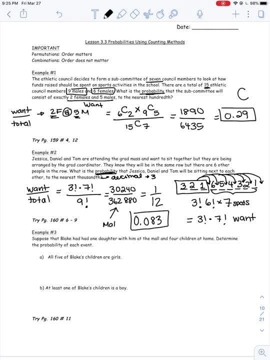 to the nearest three decimal places. so you'd have to write the answer as 0.083. so that's the answer that they were looking for. example number three: suppose that blake had had had one daughter with him at the mall and four children at home. okay, so we have with him at the mall, there is one daughter. 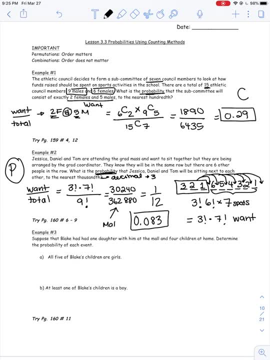 oh, and previously i just wanted to explain that in example number two. this is a permutation question, because they're being placed in seats and order matters here. this next one: here order does not matter. this is a more fundamental counting principle where we just have to use spots. so we're talking about: we have a child with him and he has. 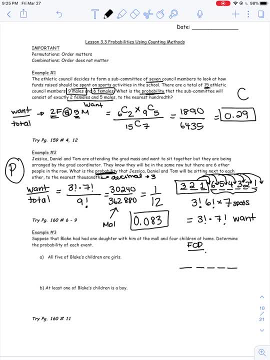 four at home. so we're gonna have four spots: one, two, three, four. since we know that the first spot, meaning the one at the mall, is a daughter, there's only one choice there, and then we have to figure out how many different options there are for the kids at home. 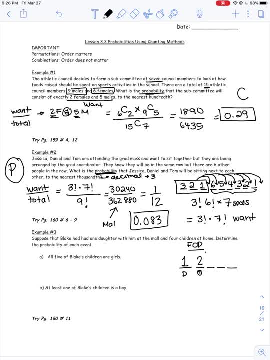 then well, let's say we talk about the first kid at home. there's two choices. it could be a boy or girl, so we would put two there. the second child at home could be also a boy or girl, so two choices. third child, same boy or girl, and fourth child at home, boy or girl. you're going to multiply all the. 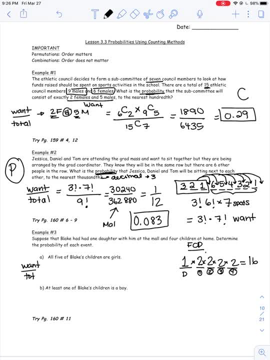 numbers and this will actually equal our total, which is 16.. so when we have our want over total, we're going to have 16 at the bottom, because there's 16 different outcomes that can occur. now we want to figure out how many ways can all five of blake's 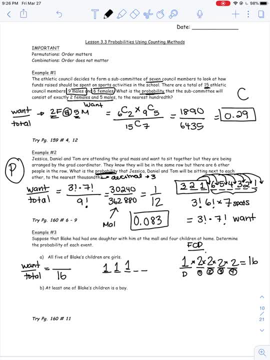 children be girls. well, there's five spots. we know that the first one's going to be a girl, the second one's going to be a girl. the third one's going to be a girl. the fourth one's going going to be a girl. The fifth one's going to be a girl. If you multiply all these numbers, you get: 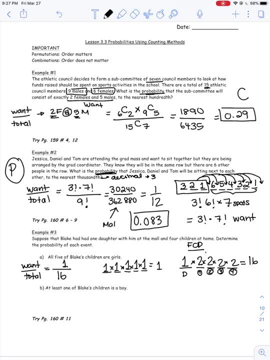 one. There's only one out of 16, um 16 possibilities that you will have all of Blake's children being a girl being girls. So that's your answer. Now, at least one of Blake's children is a boy. At least means that you could have um one child being a boy, two children being a boy. 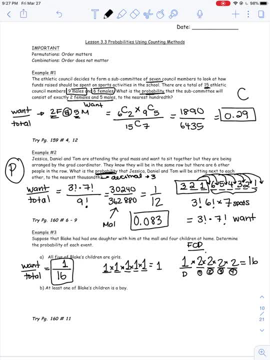 three, four, five, all the way up right. So there's a lot of options. We're going to actually use that indirect reasoning idea. It makes it way easier to solve a question like this, Reason being that the total meaning all. 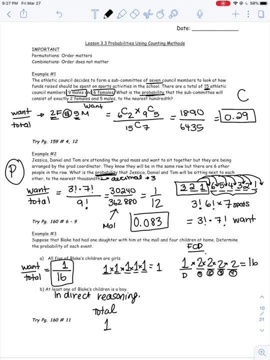 cases should always add up to one. If we're talking about fractions or decimals, or if we're talking about percents, it would add up to a hundred percent. So we know that the total is one. We're going to subtract from it. the opposite of this case. If we know that, we 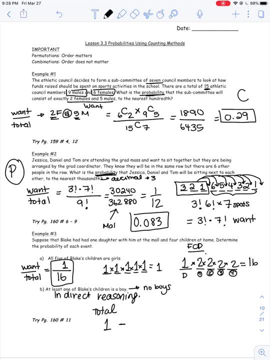 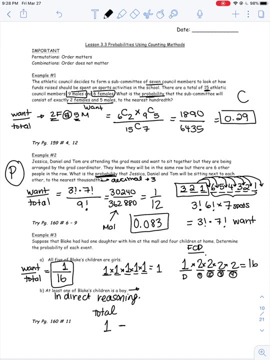 want to have a boy. well, what if we had no boys? That would be like that uh, indirect reasoning where we're taking no boys and subtracting it from our total And that's going to give us every oh sorry, no girls. It should be over here. If I fix this, this should actually be no girls. 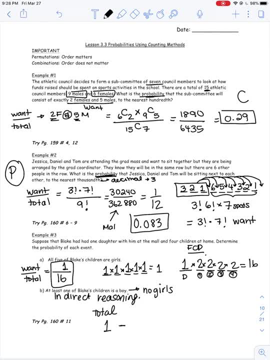 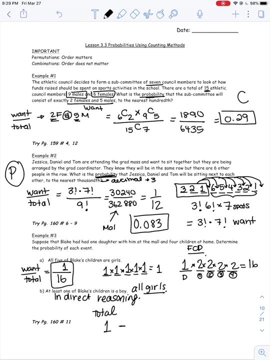 If I want to have a boy in it. the indirect reasoning, the opposite of that- would be: oh okay, Oh yes. So the indirect reasoning for this would be: what? if they're all girls, All girls, There you go, All girls, Okay, That's better. So remember, if we have one boy, two boys, three boys, 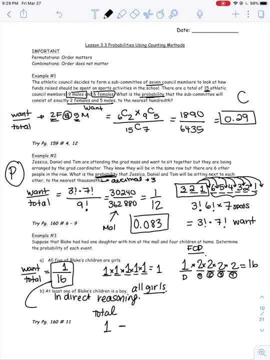 there's never going to be a possibility that there's all girls, So that would be what we have to subtract. So what you're going to do is take this answer and you're going to subtract it from one. You're going to go one over 16, subtracted from one If you're doing fractions. 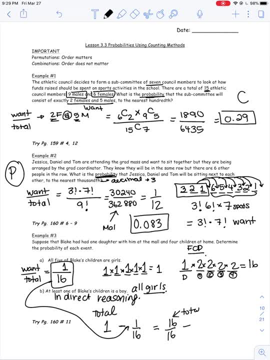 you always want to get the same common denominator. So 16 over 16 is the same thing as one, And what we're doing. so this is still our total Instead of one. we're writing 16 over 16.. We're subtracting the time. 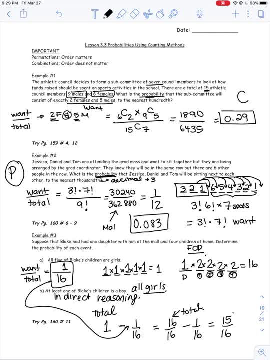 where there is all girls, which is one time out of 16.. And then that means that every other case- meaning 15 cases out of 16, will have at least one boy. So that's our answer, So indirect reasoning. we took one subtracted where all of them were girls and we got every. 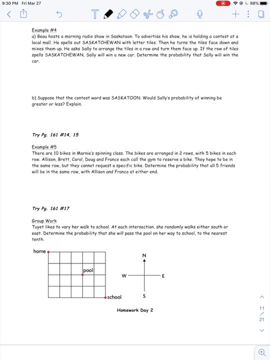 case where there were all girls. So that's our answer. So, indirect reasoning, we took one that would be a boy. Example number four: So Bo hosts a morning radio show in Saskatoon. to advertise his show he is hosting a contest at the. 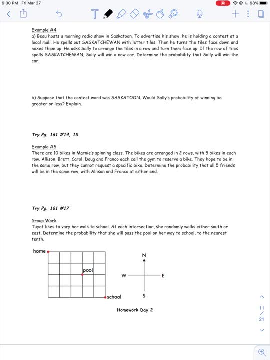 local mall. he spells out Saskatchewan with letter tiles, then he turns the tiles face down and mixes them up And asked Sally to arrange the tiles in a row and turn their face up. If the row of tile spells Saskatchewan, Sally will win a new car. Determine the probability that Sally. 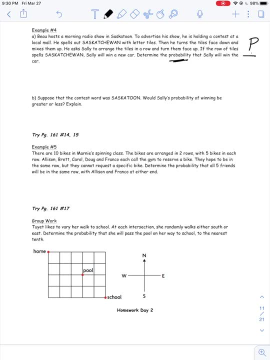 will win the car. Well, this is a permutation question, because order matters. If you turn the letters over and it doesn't spell Saskatchewan, you mix the A and the S together or the A and S spots, then it's not going to, you're not going to win. So order does matter. 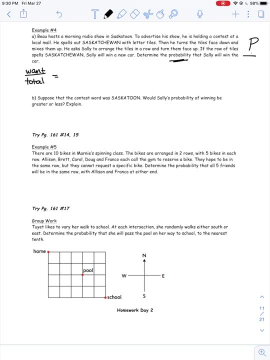 here. So we're going to figure out our total. Remember it's always going to be want over total when we're talking about probability. Our total is going to come from rearranging the letters of the word Saskatchewan. Well, whenever we rearrange letters of a word, we count how many. 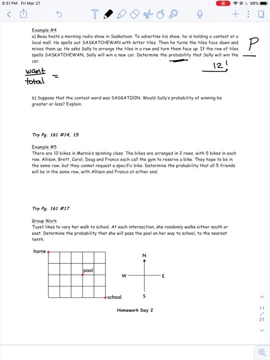 letters there are. There are 1,, 2,, 3,, 4,, 5,, 6,, 7,, 8,, 9,, 10,, 11,, 12 letters in the word Saskatchewan. So I would have 12 spots with 12, then 11,, 10,, 9,, all the way down. Now, if there was no repetition, 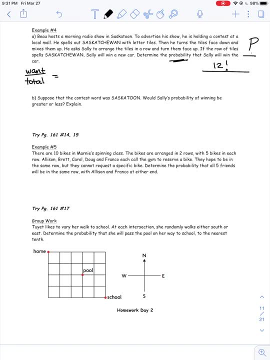 meaning no letters that were identical. this would be my answer for the total. But we actually know that there are two S's and there's actually three A's, So you want to check to see if there's any other things. So we got no more K's, no more T's, no more C H E W A N. So check that there's no other. 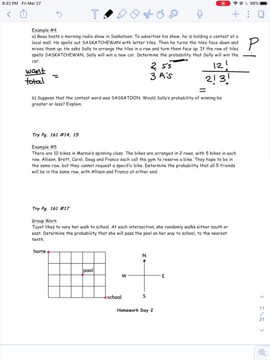 things. So what we need to do is, with the 12 factorial, we need to divide out 2 factorial and 3 factorial And you put that in your calculator with brackets around it. if you're doing it in one step And you should get 39916800. Okay, so your total will be that number. 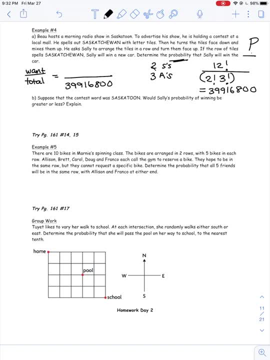 Now we have to figure out how many ways are there to turn over the tiles and spell Saskatchewan. Well, if we get rid of the repetition, just like we did before, there should only be one correct way, So there's only one correct answer. 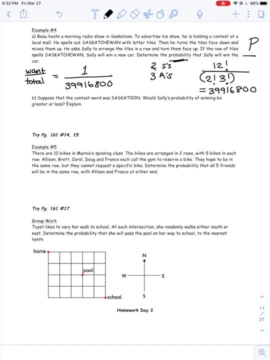 Okay, so only one correct answer needs to be done for the top. The want is to spell Saskatchewan one way, And then there's a lot of ways to rearrange the letter. So that was where we got that big number at the bottom. Now, what if you have Saskatoon? So let's figure that. 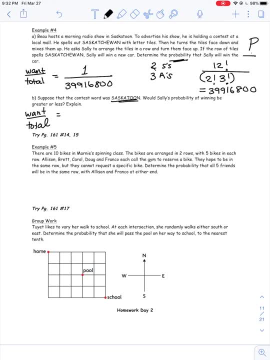 out Want over total. We're talking about probability. We would do a similar thing, we would count how many letters there are: 123456789.. So it's nine factorial divided by repetition. There is two factorial meaning the two S's, there's two A's and there's two O's. 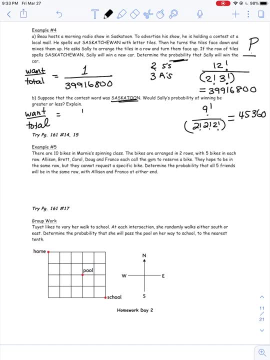 put brackets around it. if you're putting in your calculator, you should get 45,360.. So, just like in the previous case, there's only one way you could spell Saskatoon over 45,360 different arrangements. Now, from this we would find out that Sally's probability of winning would be greater in this. 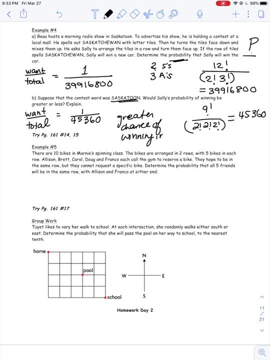 case versus A, So she has a greater chance of winning in B, The reason being: when your number, your total number, is smaller, then you have a better chance of winning. Example number five: So there are 10 bikes in Marnie spinning class, So we have 12345.. And there's two rows 12345.. 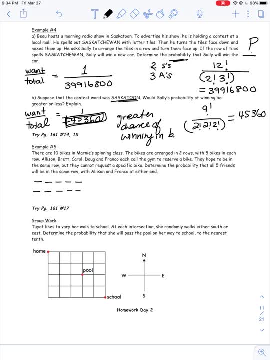 With five bikes in each row. Alison, Brett, Carol and Doug and Franco each call the gym to reserve a bike. they hope to be in the same row, but they cannot request a specific bike Determine the probability that all five friends will be in the same row with Alison and Franco. 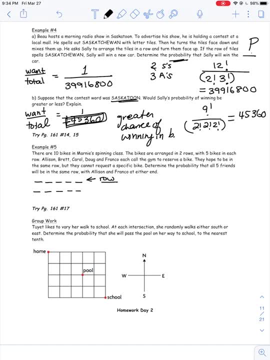 on either end. Okay, so we want Allison and Franco on either end. So let's say they're in this row. we're going to place them now in this row. If Allison and Franco have to be on either end, we can make Allison and Franco go here and whoever's left will go in the last spot. So 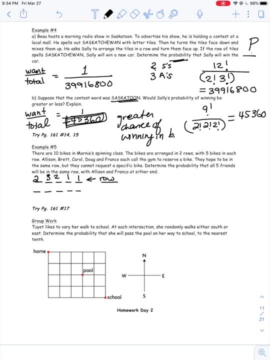 there's two: one to rearrange Allison and Franco, And then there's three- two one left over because Brett, Carol and Doug have to still be placed Now we still need to remember that there are other people that have to be placed as well. There are five other people attending this class. 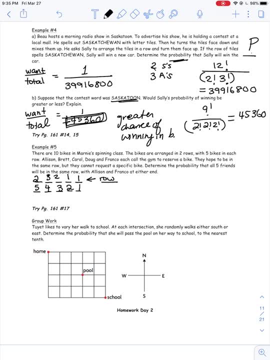 So we could have five, four, three, two, one. Okay, so what we're doing is we're writing two factorial, which represents Allison and Franco. Franco, this is, this is our want that we're creating right now. Right now, multiplied by there's three other friends, Brett, Carol and Doug, that have to be: 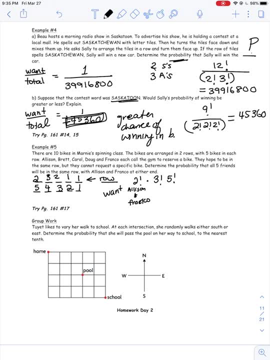 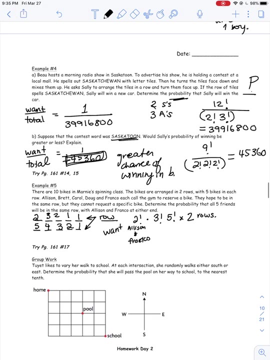 placed Now. then there's the five other people that are strangers to them, that have to be seated in the other row, that have to also be rearranged, And finally they could go in this row or this row. So we're going to have to multiply this whole answer by two, because there are two rows. 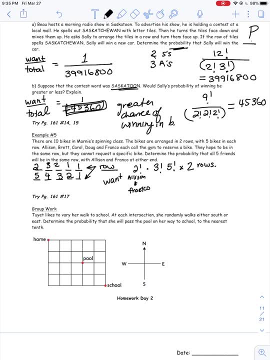 So this is our want here that we're creating. So you would put that into your calculator: two factorial times three And you should get 2880. Okay, so check that you're getting that number. I'm just triple checking. Yep, Okay, And the bottom would be your total. your total would be well, what if there were no? 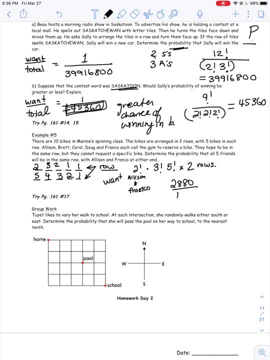 rules. There's just 10 bikes and I have to rearrange 10 people that are going to be coming to this, this spin class, So I would just go 10 factorial. 10 people rearrange is 10 factorial. So that would give you in your calculator. 10 factorial would be equal to: 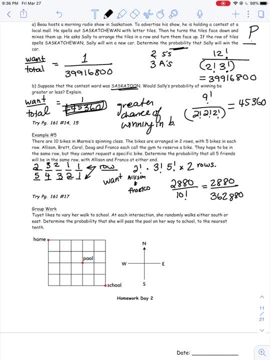 362 8800.. So it'll be 3 million 628,800.. Now, finally, we want to simplify by going math, enter, enter, and you should get that this number is nine over 11340.. Okay, so that's going to be. 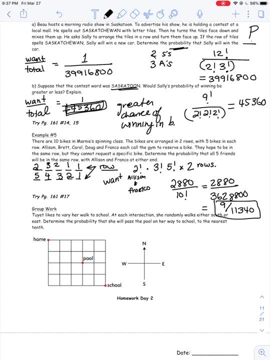 nine over 11,340 as your answer. So if they don't tell you that they want to the nearest hundredth or 10,, 10th or 1000, you can leave it as a fraction, if you want, as your final answer. 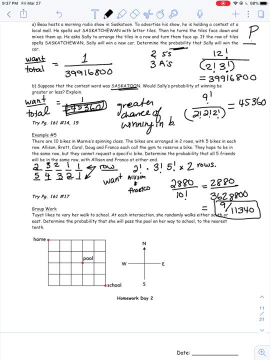 Okay, our next case is those block ones. So what we're going to have to do is a finder total, So our total would be going from home. it says we're going to need this for school. Oh, and we're not going to need this because we already do a square, so something like that. 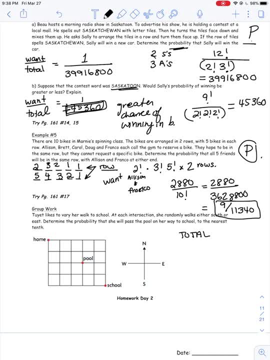 but for now we'll leave it as square because we don't want to lose the question this way. So we're going to say a lot of times: we don't need this, because we don't want to lose the question this way. So I'm going to give you this as a final answer. 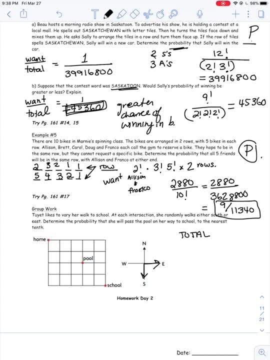 So I'm going to go with the last one. So I'm going to go with in check. I'm going to go with in check on our way to school. Well, first we need the total. The total would be going from home to 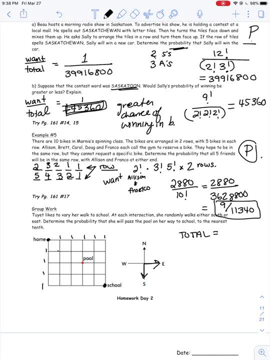 school without having to go and pass the pool. So back in the day we put ones ones, ones, ones along the edges and then we would add up: one plus one is two, Two plus one is three, Three plus one is four, Four plus one is five. Five plus one is six, And then one plus two is three, Three plus. 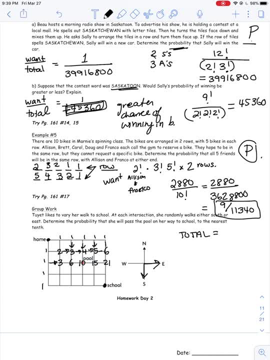 three is six. Six plus four is 10.. 10 plus five is 15.. 15 plus six is 21.. Three plus one is four. Four plus six is 10.. 10 plus 10 is 20.. 20 plus 15.. 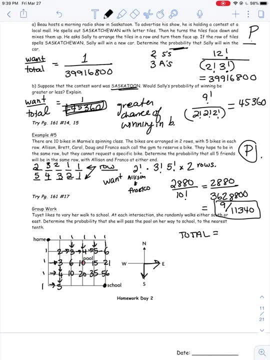 15 is 35.. 35 plus 21 is 56.. Then we have four and one is five. 10 and five is 15.. 15 and 20 is 35.. 35 and 35 is 70.. And then 70 and 56.. I'll go to my calculator: I get 126. 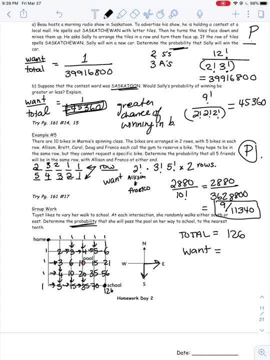 So I know my total is 126.. Whenever you're trying to find probability, you still need to figure out the want, And in our case the want is going through the pool, So want is going through the pool. So I'm going to erase this. 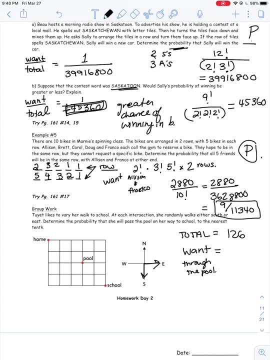 and start all over again. So again we can only go right and down, but we have to go through this without going past it and then through here. So it's kind of going to look like this, because here, if I go to this next spot right here, I would not be able to go down and go through the. 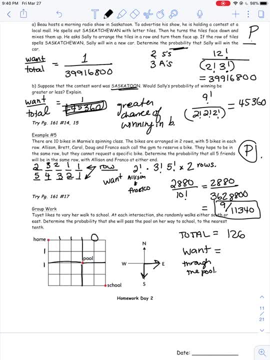 pool. So it doesn't make sense to go past the pool either horizontally or vertically. Okay, so along the edges I should have ones then. one plus one is two. two plus one is three. I don't want to go lower because then I won't go through the pool. Two plus one is three. three plus one. 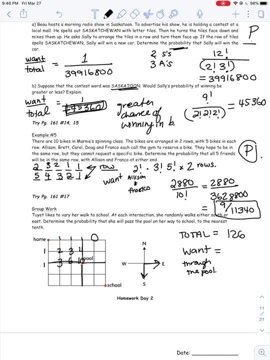 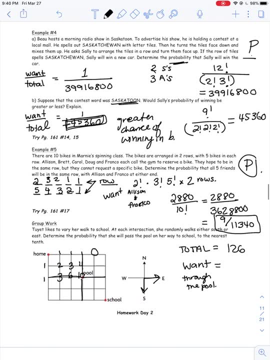 is four. three plus three is six. six plus Four is 10.. So now I'm going through the pool Again. I don't want to go anywhere outside of that box that I created, because that would be going backwards or up when I should be only going. 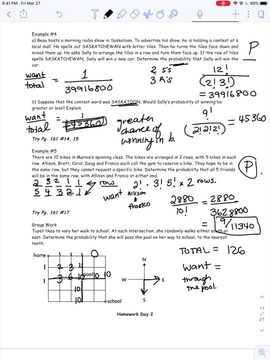 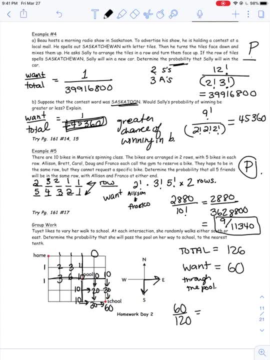 and then 30 plus 30 is 60. So that is our want. So we're going to have 60 over 120, which we'll put in our calculator because it does want the answer to the nearest 10th. So that would be 0.5 if you round to the nearest 10th. 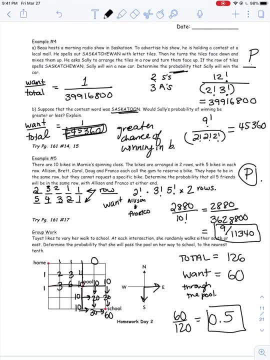 Okay, so that is lesson 3.3, using counting methods. So this is kind of reviewing permutations, combinations In order to answer the question. The reason this is different than our previous lesson is just because of this word. This word changes what we're doing.